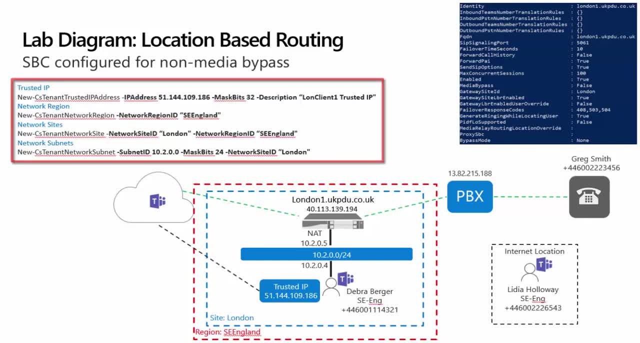 a site called London and the subnet, or subnets of the site. I also have two users, Deborah and Lydia, who are enabled for Locations-Based Routing, which are associated with my London site. In my configuration, the London site is enabled for. 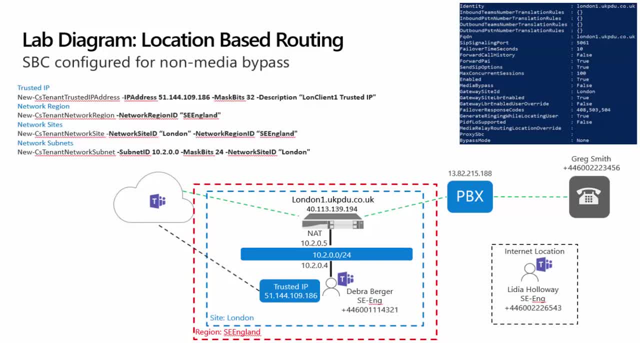 Locations-Based Routing. Locations-Based Routing is relatively straightforward to configure, but in my opinion its operation is actually very complex and multiple call scenarios, such as basic call transfers and delegation, will be impacted. Throughout the rest of this video, we will look at a few example call flows. 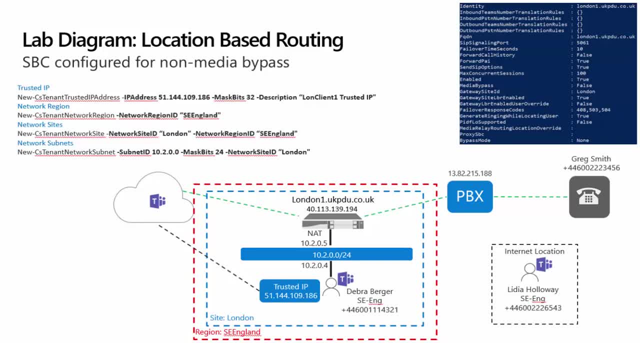 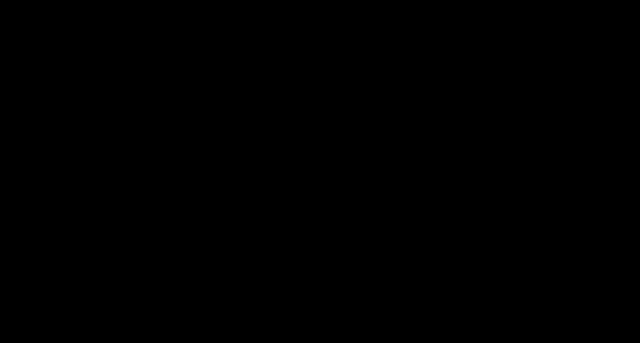 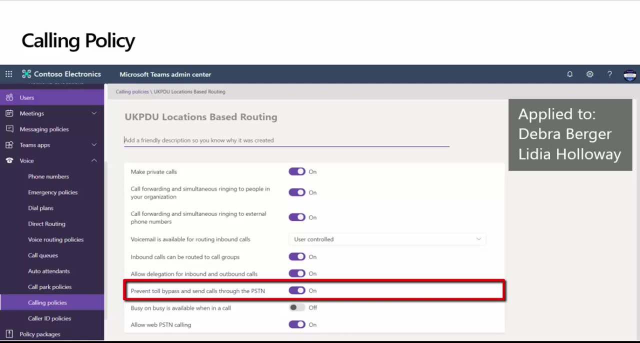 but you are highly encouraged to review the Microsoft documentation that provides a thorough explanation of how calls will be routed based upon a user's location. As shown, the calling policy that enables Location-Based Routing is called Prevent Toll Bypass and send calls through the PSTN. In my lab, the UK PDU Locations-Based 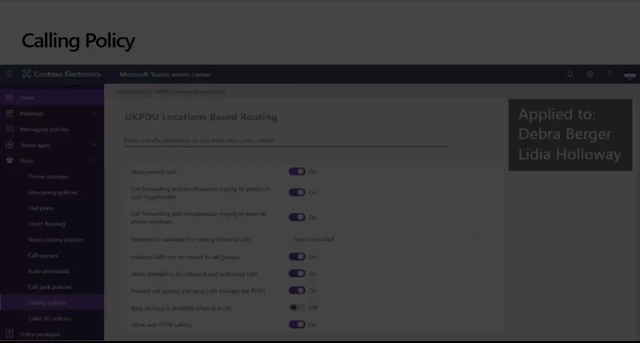 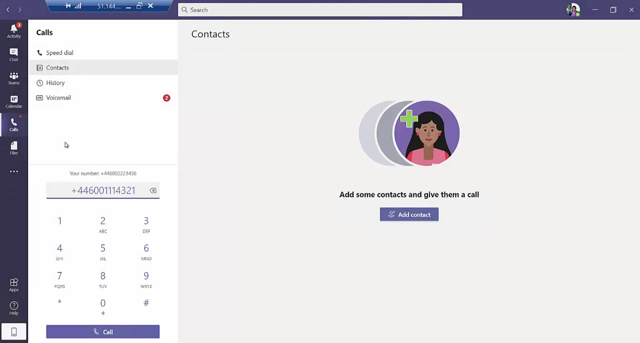 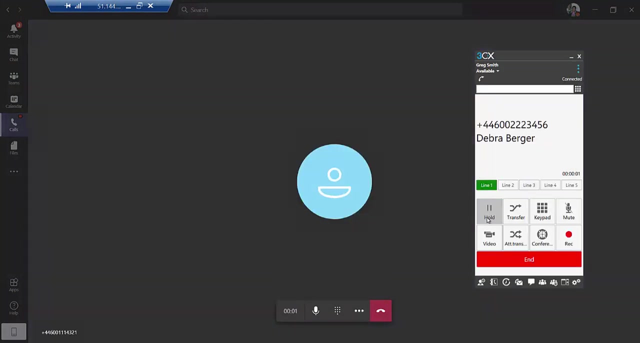 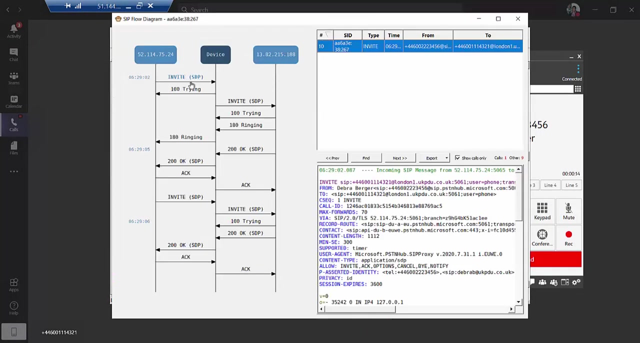 Routing policy is assigned to Deborah and Lydia. In this first example, Deborah calls Greg. As Deborah is in London and her call plan includes the London SBC, her outbound call is successful. Note that because the SBC is configured for non-media bypass, 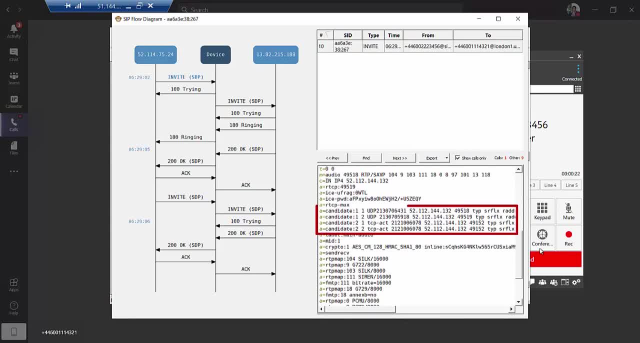 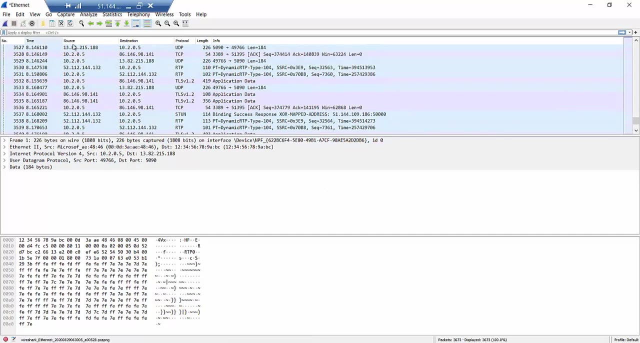 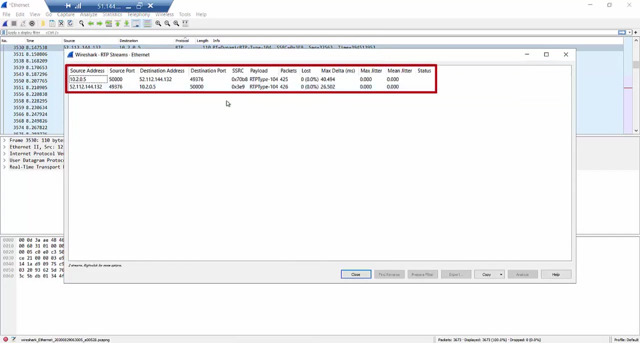 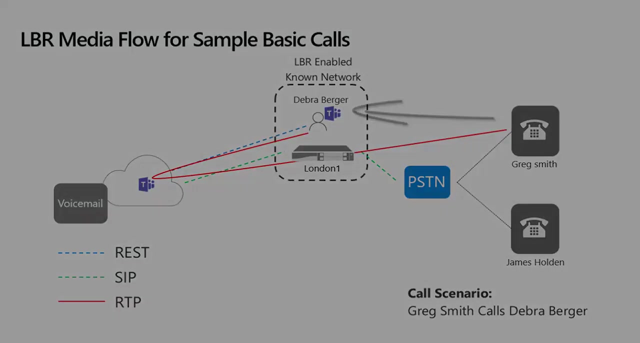 the media flow that's negotiated via the SIP, ICE candidates will traverse the Microsoft Cloud. When she calls Debra, the incoming PSTN call will arrive at the London SBC. The call has been successful, but it also includes two different RTP calls that will be used to. 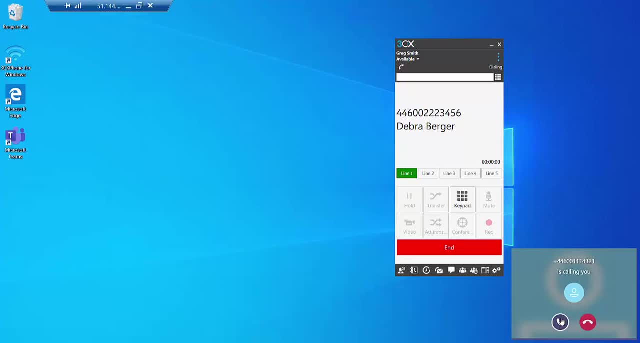 signal the London SBC Again, because Deborah is in London, Toll bypass won't occur, so the call is createable. What we can also see is that in the RTP Sniffer Trace. we can also see this in the RTP Sniffer Trace.